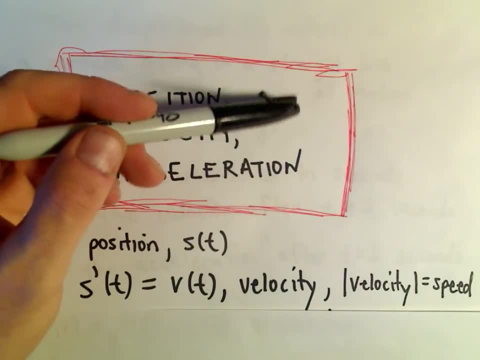 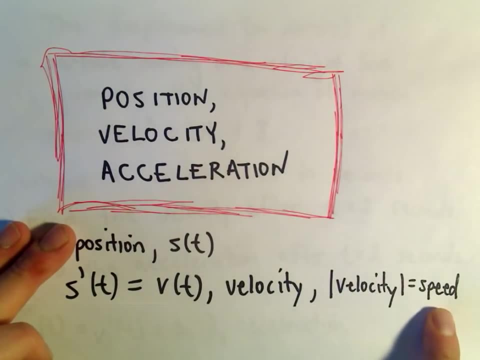 And if you're velocity? If your velocity is positive, that indicates you're moving away from home. If your velocity is negative, it indicates you're coming back To get speed. speed is always positive, So all we really have to do is just take the absolute value of velocity to get our speed. 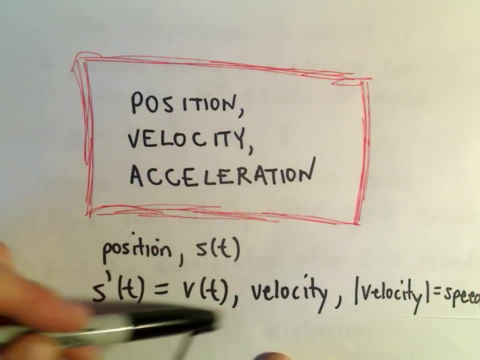 Well, if we calculate the instantaneous rate of change of velocity, well, when we take the derivative of velocity, that tells us about acceleration. So the derivative of velocity, which would be the second derivative of our position, That's going to tell us about acceleration. 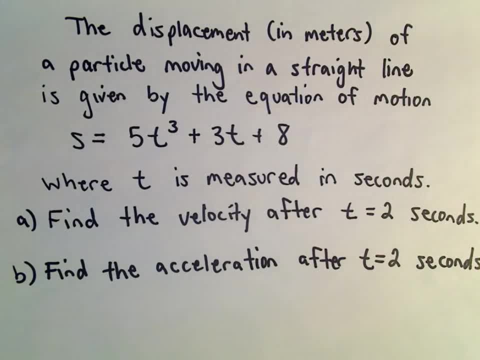 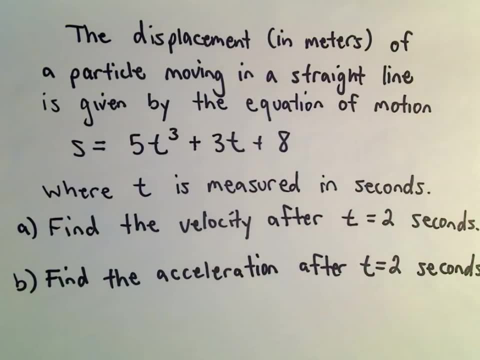 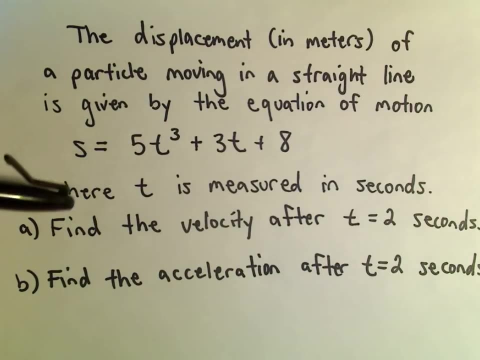 So let's maybe do kind of one mechanical problem and then I'm just going to talk a little bit for a second. why this? hopefully, why this makes sense. So the displacement in meters of a particle moving in a straight line is given by the equation of motion s equals 5t cubed plus 3t plus 8, where t is measured in seconds. 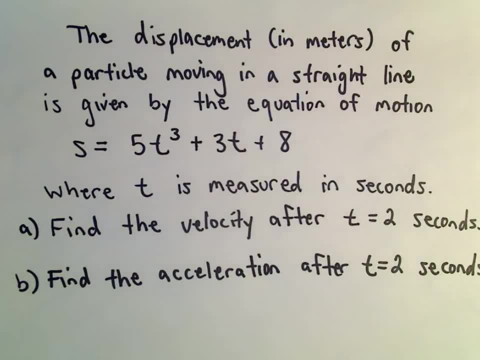 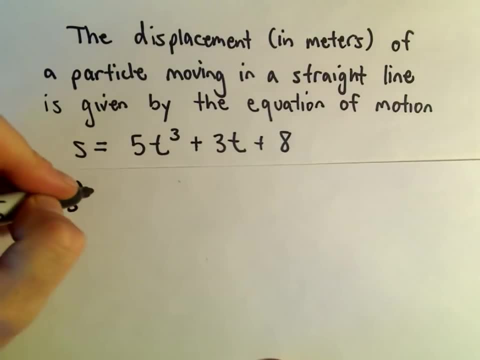 We want to find the velocity after two seconds and then the acceleration after two seconds as well. So all we have to do is just take some derivatives, So the derivative of our position function, and we can even stick a t in there if we want to. well, that's going to be the same thing as our velocity equation. 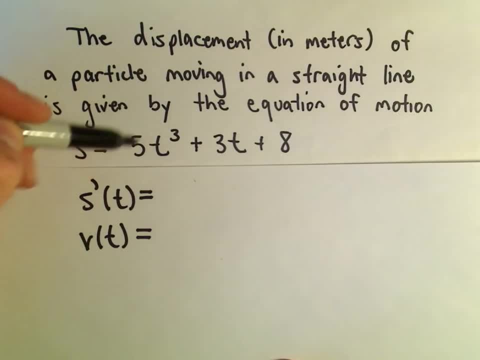 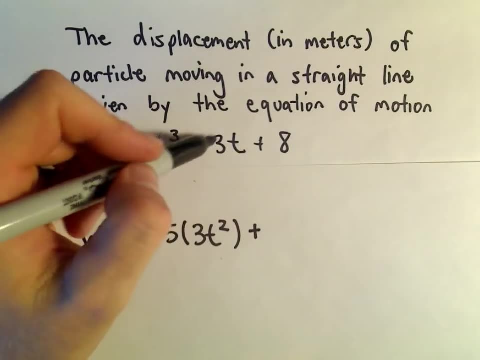 Well, if we take the derivative of 5t cubed, the exponent would come down front, so we would have 5 times 3t squared. The constant just kind of comes along. The derivative of 3t is simply 3, and the derivative of positive 8 is 0. 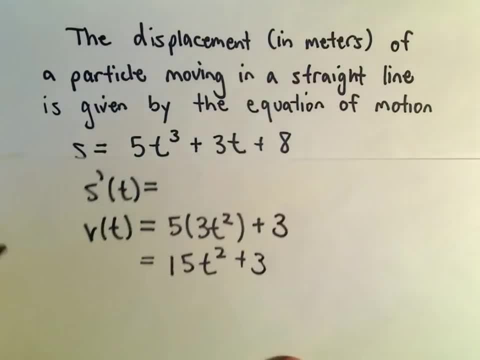 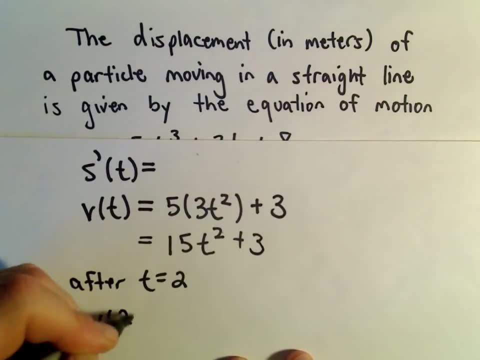 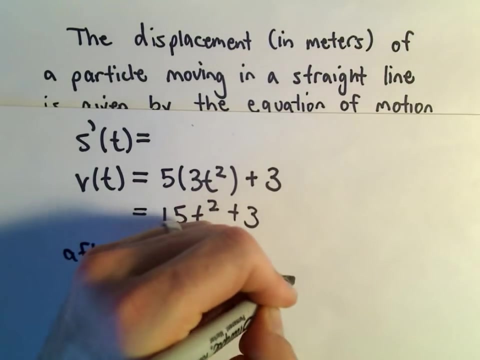 So we'll get 15t squared Plus 3.. Well, that means the velocity. after well, two seconds. All we have to do is just plug it in. So if we plug in 2, we'll get 15 times 2 squared plus 3.. 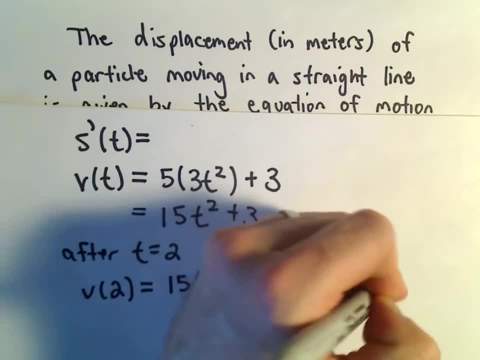 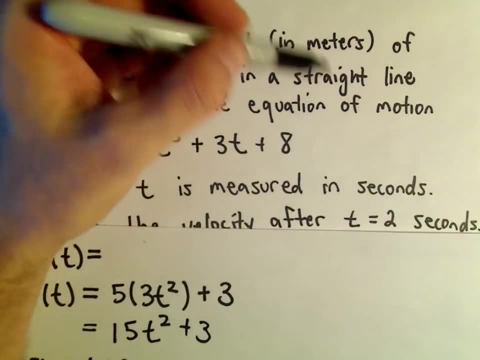 2 squared is 4, so we'll get 15 times 4 plus 3.. 15 times 4 is 60, plus 3 will give us 63.. And it was in meters and seconds. Those were our units. 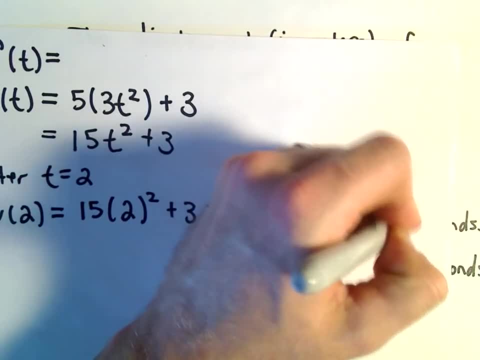 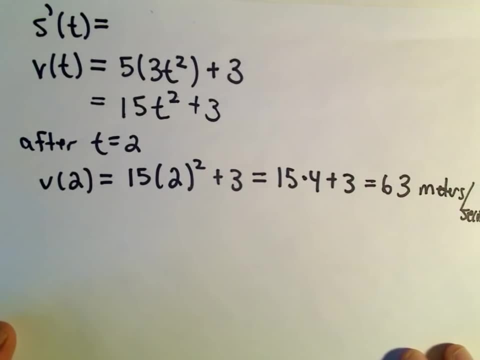 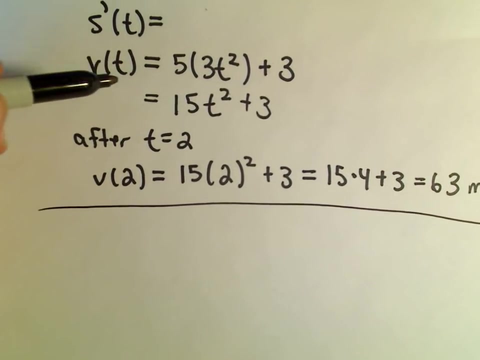 So it says your velocity. Your velocity is 63 meters per second. OK, so nothing to do, nothing tricky, nothing crazy, other than taking a derivative and plugging in t equals 2.. You know, they could ask something like: when does your velocity equal 100 meters per second? 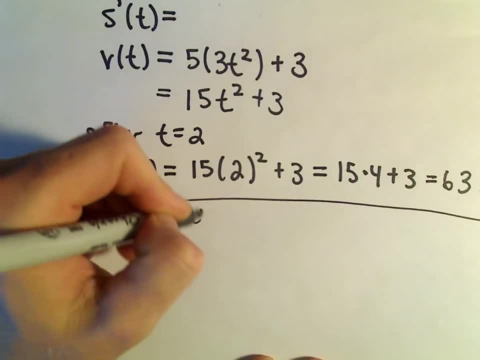 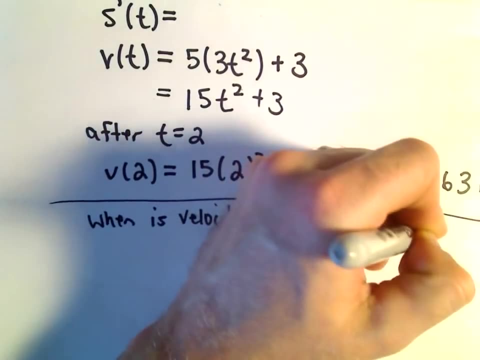 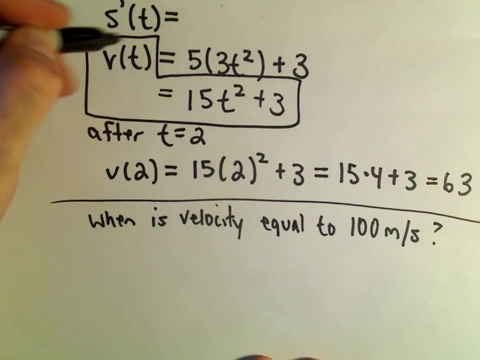 So just to throw in something different: when is your velocity equal to 100 meters per second? Well, in that case you would just take your velocity equation And now we would. we're trying to figure out when our velocity is 100. 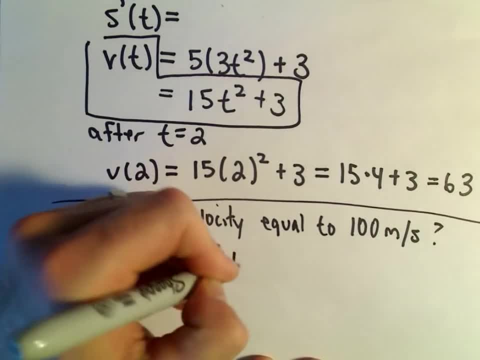 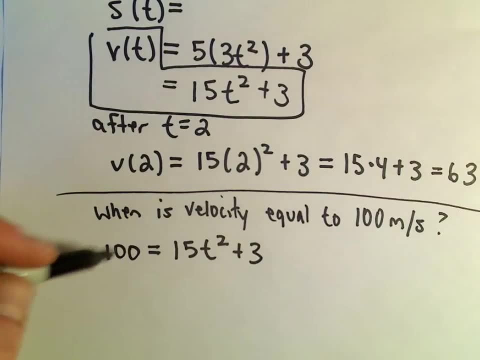 We would just plug 100 in on the left side and then you would simply have to solve for t, So you could subtract 3, divide by 15, take square roots and do all that. So I'm not going to go through it, but that's the difference. 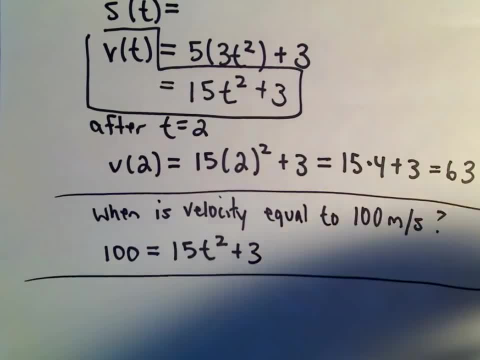 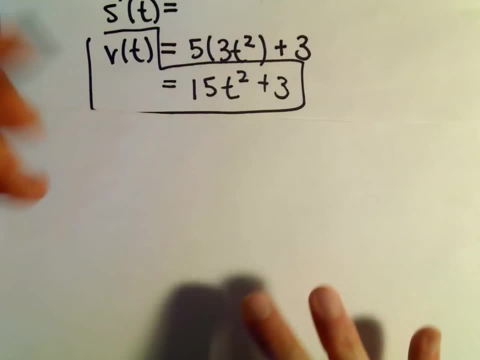 OK, you would just plug it in and then have to solve- Let's do the original other problem I did say, which was to find the acceleration. Well, again, we know our velocity here. our velocity at time t is 15 t squared plus 3.. 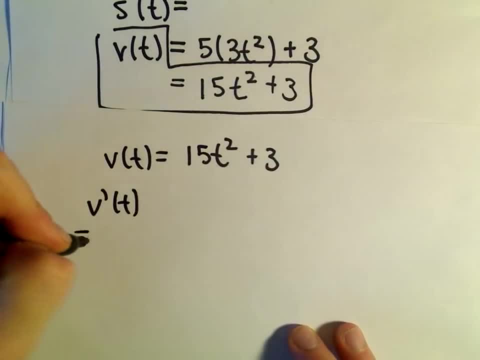 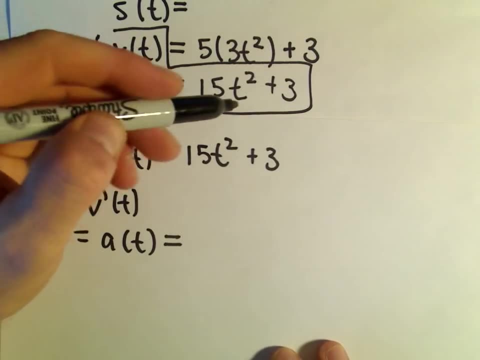 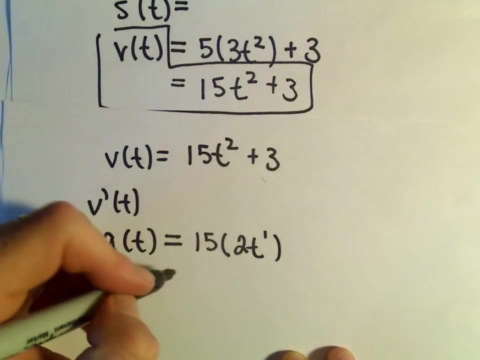 If we take the derivative of velocity, that is going to give us our acceleration function, And if we take the derivative of 15 t squared, well, the t squared will get 2t to the first. The derivative of positive 3 is just going to give us 0.. 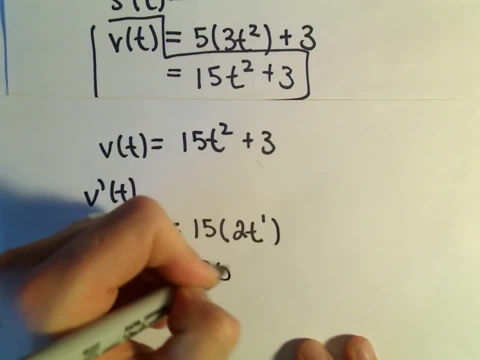 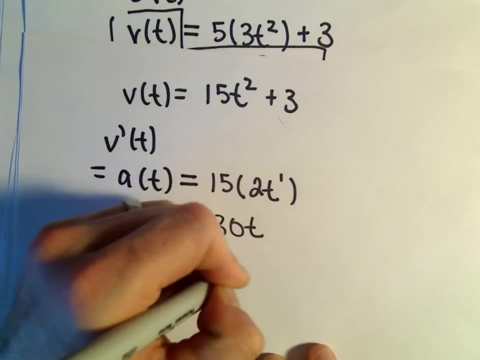 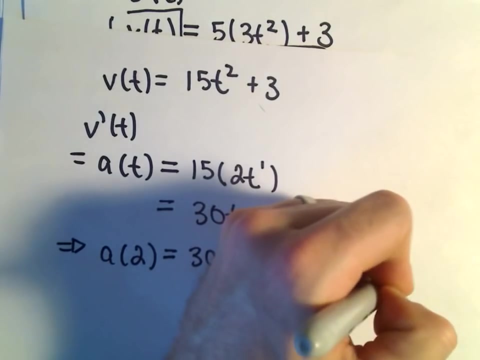 And if we multiply 15 times 2t, hey, we get 30t. So that says, our acceleration after 2 seconds would be 30 times 2.. Or we would get 60 meters, And now in the denominator we write seconds. 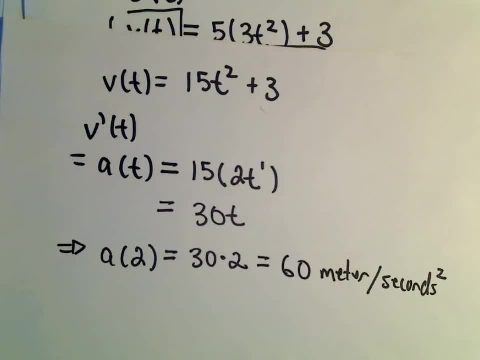 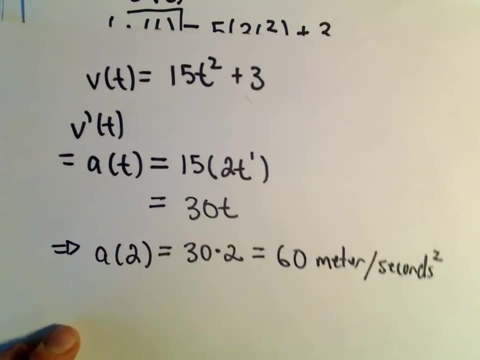 squared. OK, so those are your units: 60 meters per second, second squared. Should that be plural? I don't know. It's plural, OK, so that's the basic idea. You're just taking derivatives, is all you're doing. 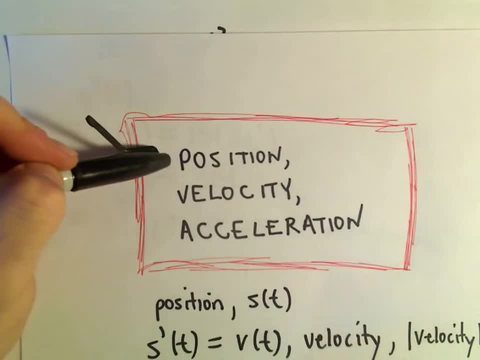 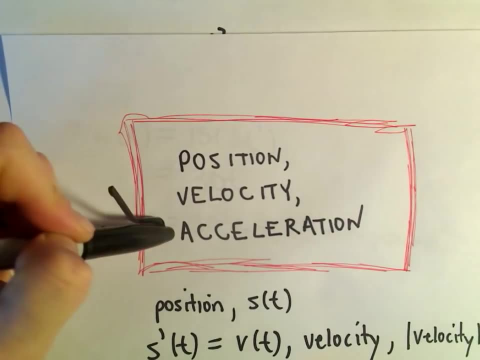 And you know. so that's the short answer. If you start with position, take the derivative to get velocity. Take the derivative of velocity to get acceleration. Equivalently, if you start with position, take two derivatives to get acceleration. 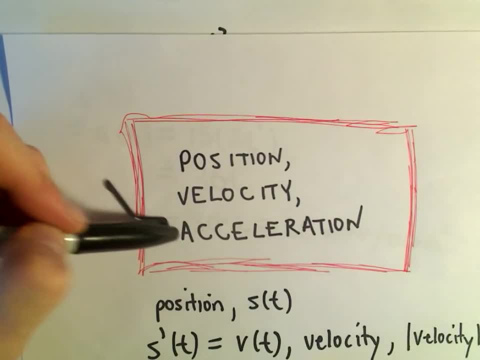 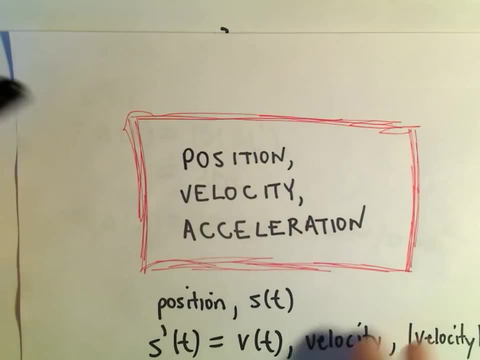 If you see an antiderivative, well, you just go backwards, you know. So if you start with acceleration, the antiderivative is velocity And then the antiderivative of that is going to tell you stuff about position. And again, why does this make sense? 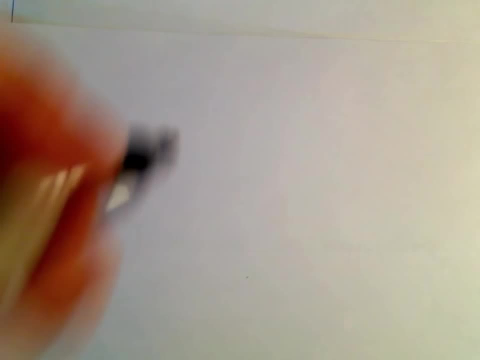 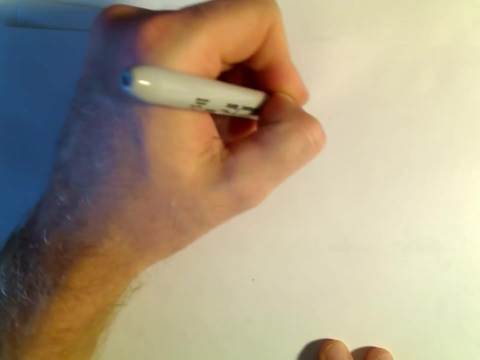 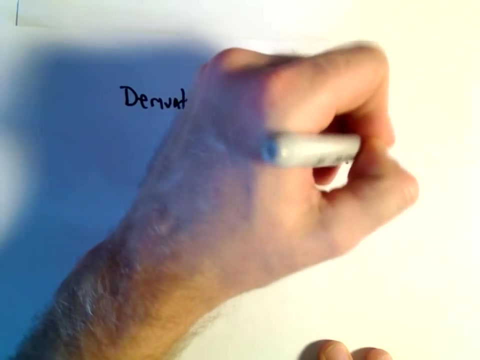 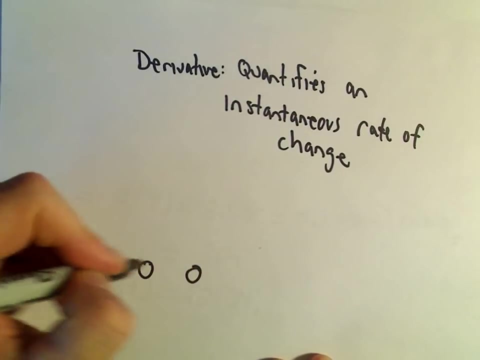 You know. so, again, a derivative, Remember, somehow a derivative. a derivative quantifies an instantaneous, quantifies an instantaneous rate of change. Well, if you're sitting in your car, right, and you're driving along, I'm going to try to draw a terrible little car. 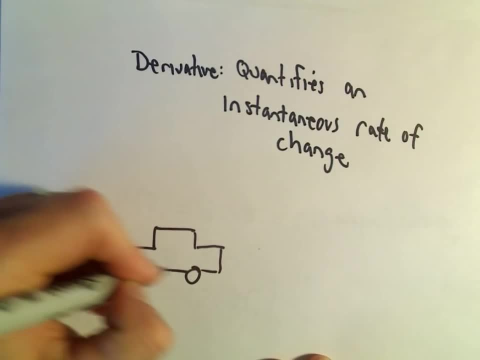 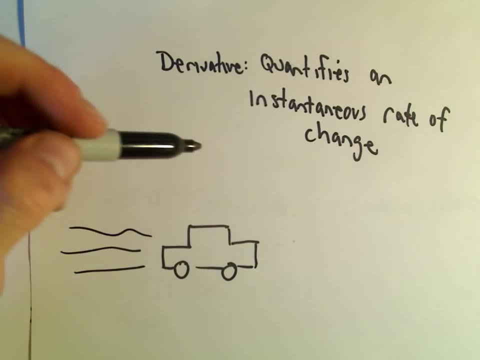 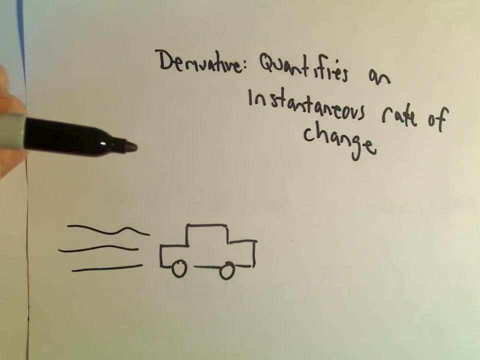 Um, Hey, that's a great car. So if you're driving in your car, right, and you're going down the road there, if you look at your speedometer, for example, you know really that's telling you a speed, because it technically doesn't tell you. 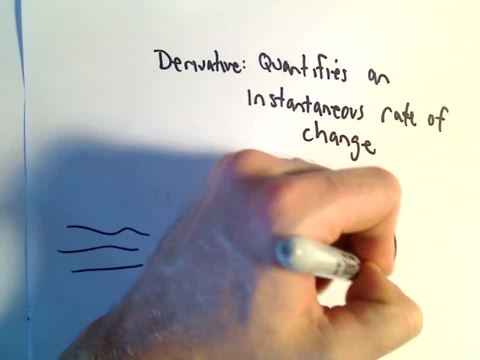 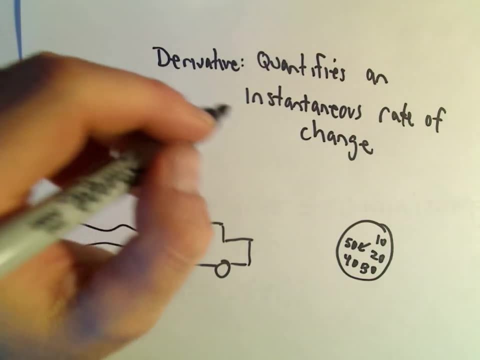 a velocity when you look at your speedometer right, Because it's not telling you the direction that you're going. It's just telling you: hey, you're going 50 miles an hour, or however fast you're going. It's a funny looking car. 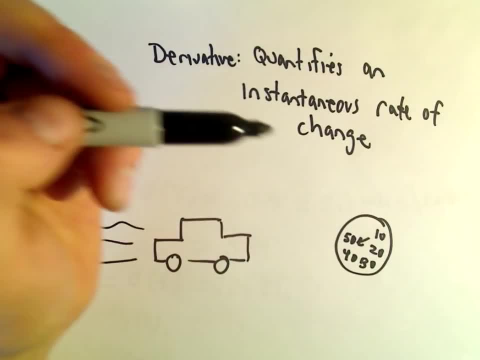 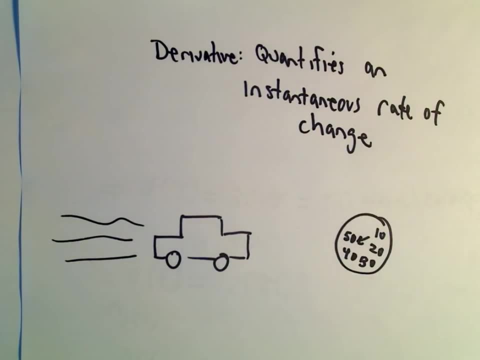 It's a funny looking speedometer. So, however fast you're going, it says you're going 50 miles an hour. Well, again, what does that 50 miles an hour tell you? It somehow quantifies the rate, the instantaneous rate. 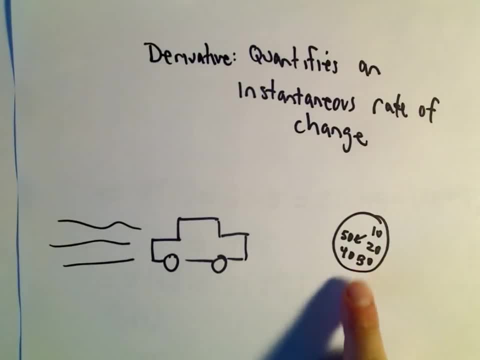 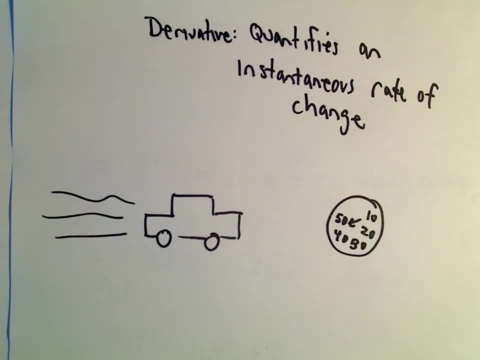 the rate at that instant. when you look at the speedometer, It's telling you the rate at which your distance is changing. So, again, if you have a function that tells you, you know. so maybe this is time T and this is your. 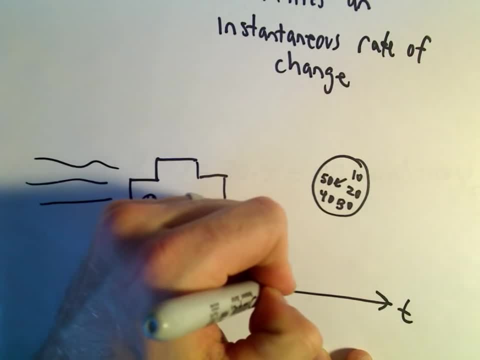 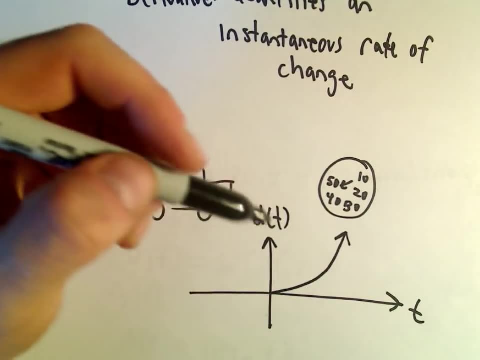 distance, maybe from home. OK, so maybe your distance, maybe you're speeding up because you want to get that. you know, get away from home really quick for some reason. Maybe you got a hot date. The idea is, if you calculate the slope of that tangent line, 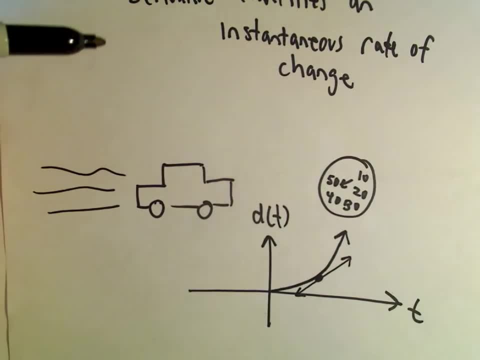 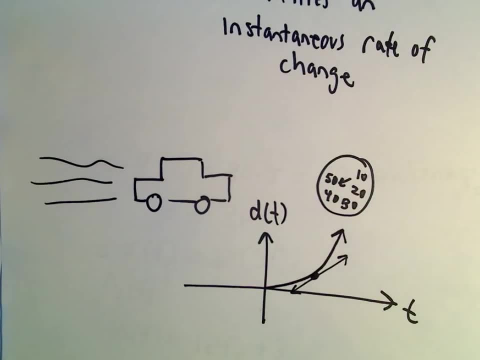 it's going to calculate the instantaneous rate of change. Or, again, it's going to tell you the slope of this line, is going to tell you the velocity. So one more time, you know when, when, you know when you're driving really fast. 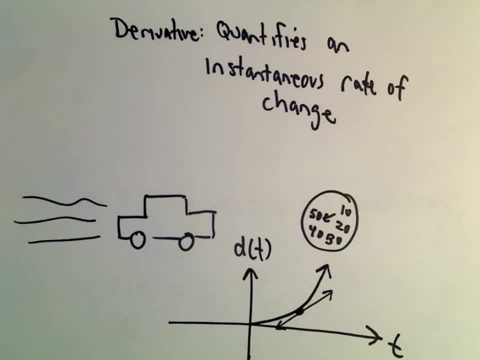 you don't say oh to your friend. You don't say the rate at which our position was changing was really big. You say our velocity, or usually you say our speed. It was really big. OK, we were going really fast. 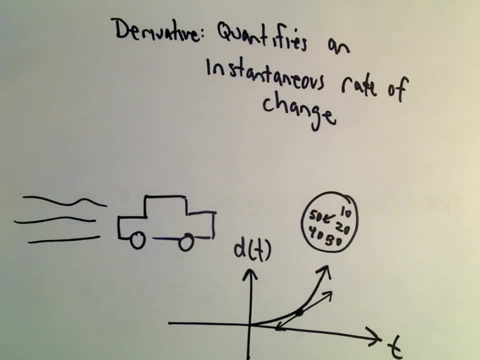 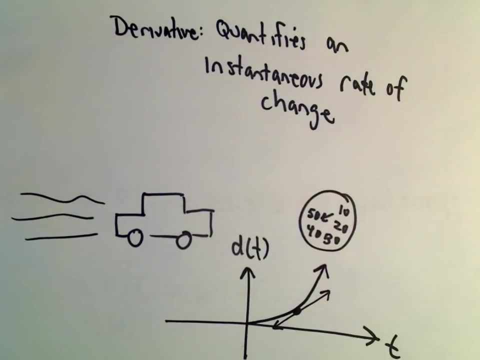 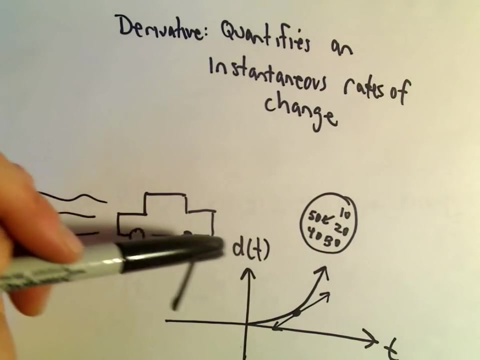 Our speed was really fast. The rate at which our position was changing was really quick, So that's the big use. Again, we talk about derivatives as being instantaneous rates of change. So, depending on the situation, what does it mean to be an instantaneous rate of change?